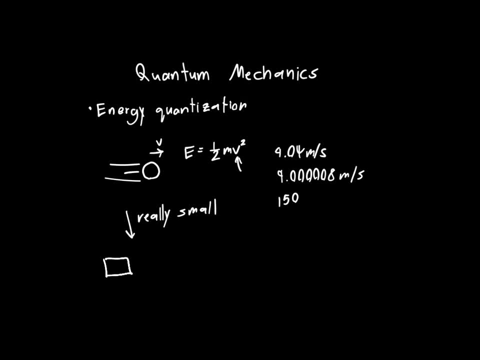 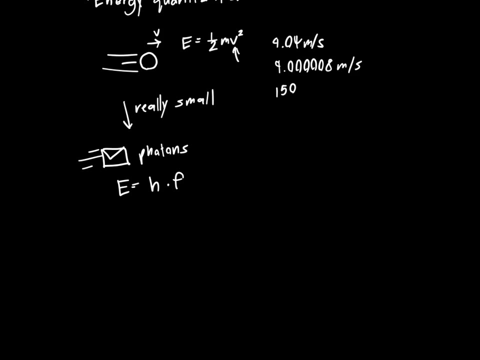 energy in individual packets called photons, and the energy of this individual packet is just h, which is Planck's constant times, the frequency of the photon f. and it turns out that this is a general formula for the energy of uh, multiple or any any particle really, in quantum mechanics. so the energy of a particle is described this way: 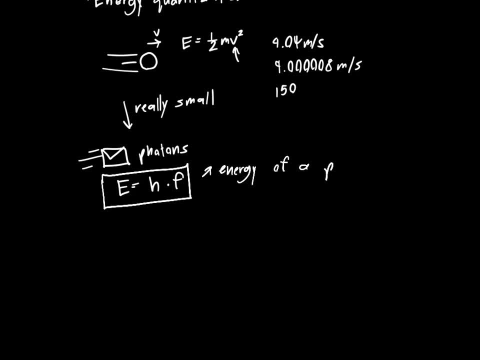 energy of a particle and uh. another postulate of quantum mechanics is that balls, uh or any, any kind of object, really aren't described by a single position. so in classical mechanics i'd have say: this ball, and it's gotten, it's got certain coordinates: x, dot, y naught, z naught- in quantum mechanics. 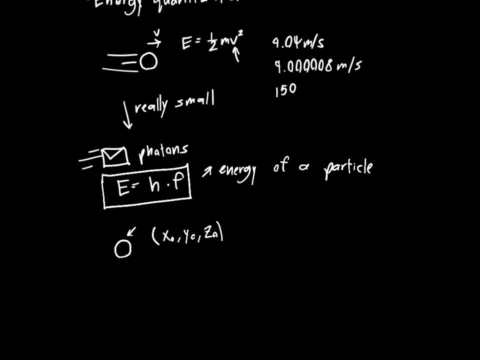 that ball cannot have a specific place. it doesn't the the? the ball itself is sort of smeared out, uh, in space. we can't say with certainty where the ball is, and that's described by the uncertainty principle, or that the delta momentum, delta x, is less than or equal to Planck's constant divided by two pi, and that 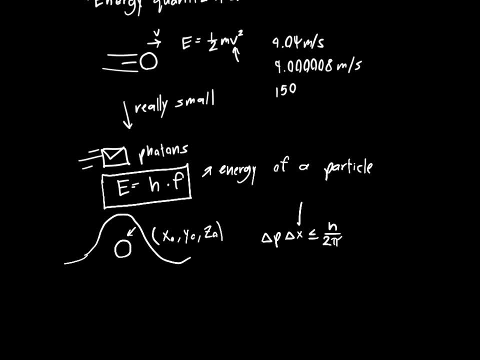 means that the position of a ball in the, in a single coordinate, is related to the momentum and we can't say with certainty. if we know what the ball's momentum is within a certain certainty, we cannot say what the position is within. so if we have delta x less than or equal, 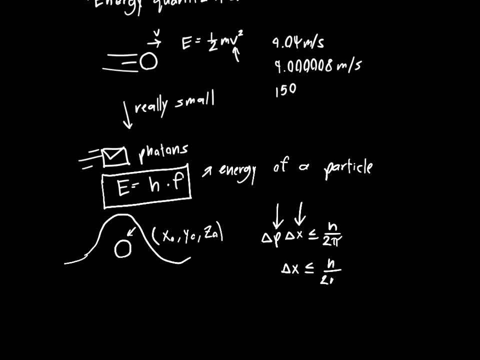 to h over 2 pi, and h over 2 pi is often called h bar, and that's actually the notation that i'm going to use. so x has to be less than or equal to h bar divided by delta p. so if we have a certain 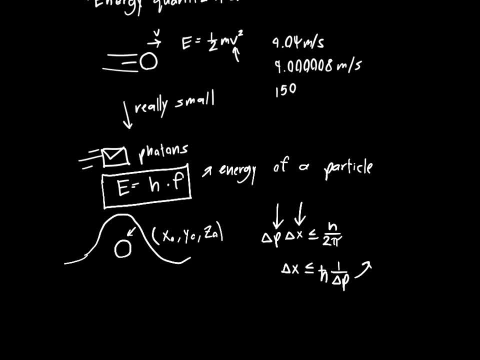 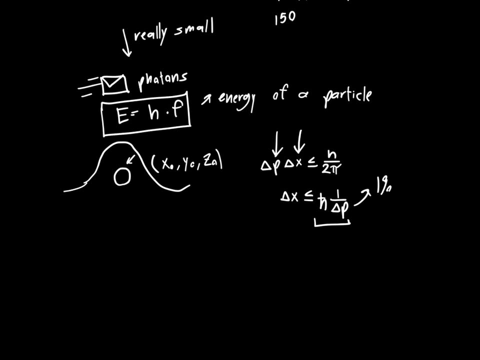 certainty of momentum. so say, we measure this within one percent, then we cannot measure x within less than h bar times one percent accuracy. so that's, that's the basic idea behind the uncertainty principle, and there's a second version of it that has to do with energy, and that's delta. 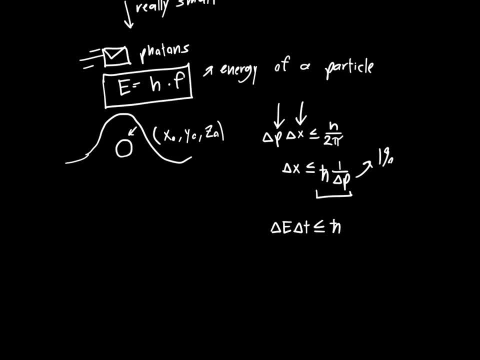 e, delta t is less than or equal to h. so if you know the energy with a certain certainty, you cannot know, uh, the particle's position in time. and this is, these are just postulates of quantum mechanics. they are true as far as we know, um, and they're also really complicated and really uh, the, the, 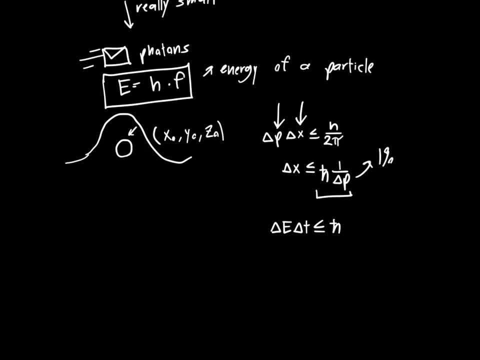 consequences are really far-reaching and we're only going to scratch the surface here. so if you're interested, i recommend you take a course on quantum mechanics, if you it's, if that's not already part of your curriculum. uh, the third postulate of quantum mechanics is that if you're interested in 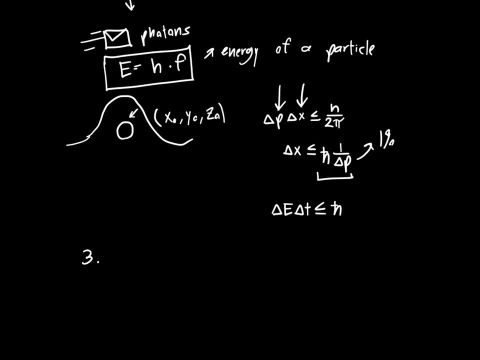 mechanics is that particles are waves or particles are not particles, but they're described by waves. they evolve in time as if they were waves, like water waves we know sort of propagate outward from a source. so if you drop a pebble into a pond, for example, the waves will radiate outward and you'll have you'll. 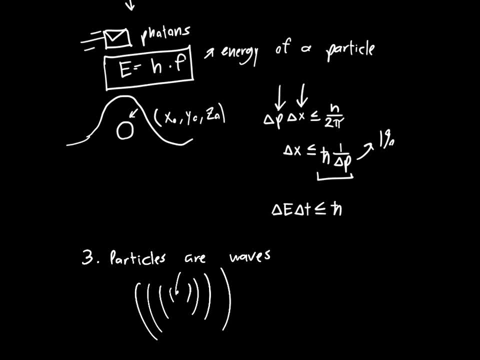 can get interference between waves and wave. waves have all sorts of phenomena that we don't typically think of as being associated with particles, but de broglie uh showed that particles do in fact have a wavelength, which is described by the equation lambda, or the wavelength of the. 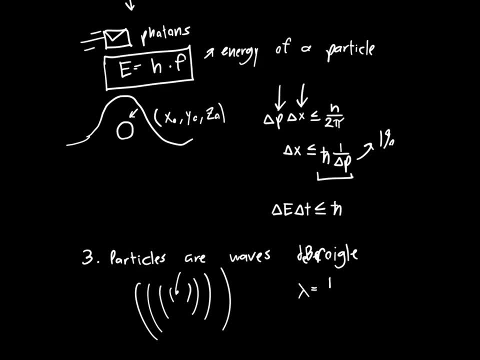 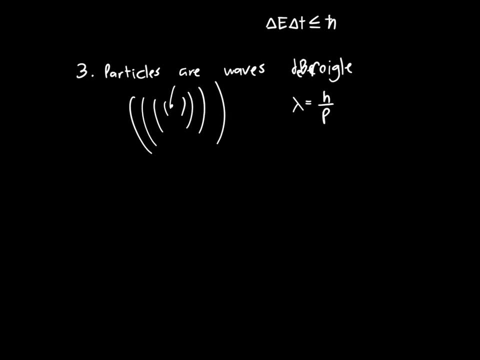 particle is equal to Planck's constant divided by the particle's momentum, and so these are the three basic postulates of quantum mechanics, and some consequences, or the ones that we're going to have to worry about, are that electrons must be described by what's called a wave function, and the wave function is often abbreviated with this: 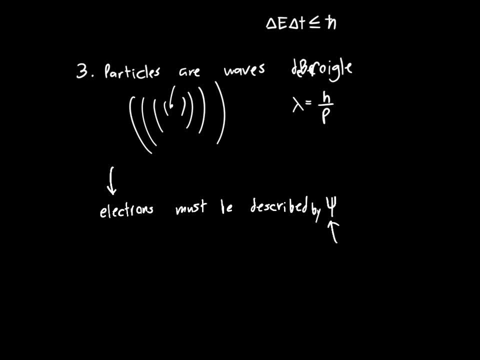 greek letter psi. and so electrons don't have a certain position. they don't really act like particles, they act more like waves often, and we can't say with certainty where the electron's position is. we can say what? the the only thing we can say actually. 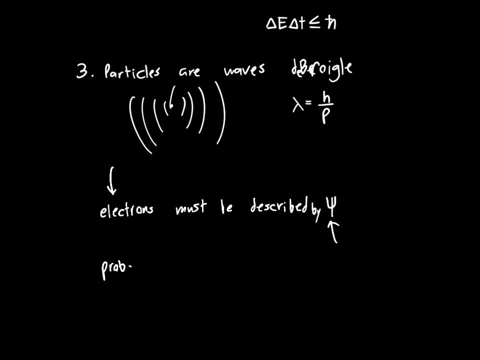 is that the probability, uh density- of the electron, or the probability that it's found at any given location, is just proportional to the magnitude of the wave function squared. and this is typically what physicists deal with when they want to make predictions about: okay, where will a particle actually end. 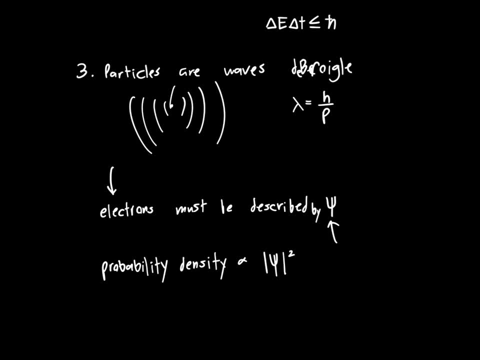 up. They deal with the magnitude of the wave function squared, And so we're going to actually solve for the wave function in the next video And then we're going to take the magnitude squared and we're going to see where particles are actually located or where an electron is located. 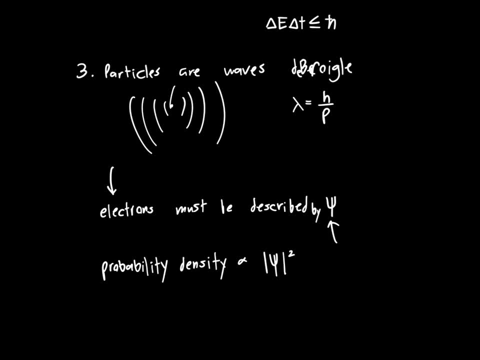 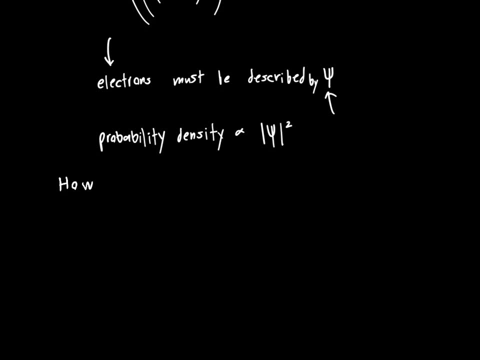 with certain probability. So there's one question that you might be having, and that's well, that's all great, but how do I do quantum mechanics? So we can make these postulates, we can say all the interesting things we'd like, but how do we actually use it to solve engineering problems? 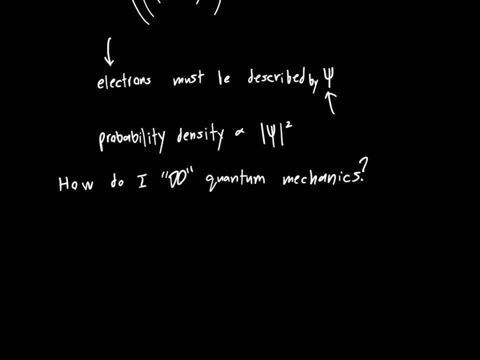 And the answer is in the Schrodinger equation, And you might have seen it in various forms, but I'm not going to go into that, So I'm going to go into it in a little bit more detail. So I'm going to go into it in a little bit more detail, And I'm going to go into it in a little bit more detail. 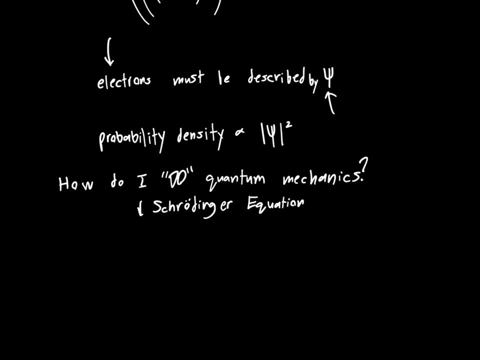 I'm going to write it in a form that I think is the most friendly. So the Schrodinger equation is actually going to take one of two forms. The first one is d squared y, dx squared, where x is your coordinate, x is some coordinate and y is the wave function is equal to minus k squared times y. 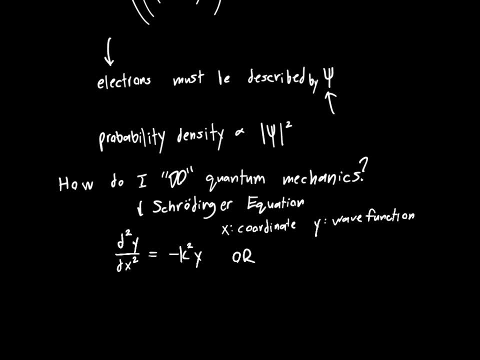 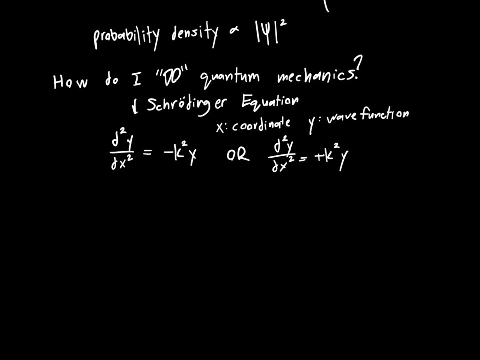 or sometimes it'll appear as d squared y. dx squared equals plus k squared y, And so the Schrodinger equation will always be in well, I should say, for the things we'll be using it for. it'll always end up in one of these two forms, And we actually know the solutions to these differential equations.